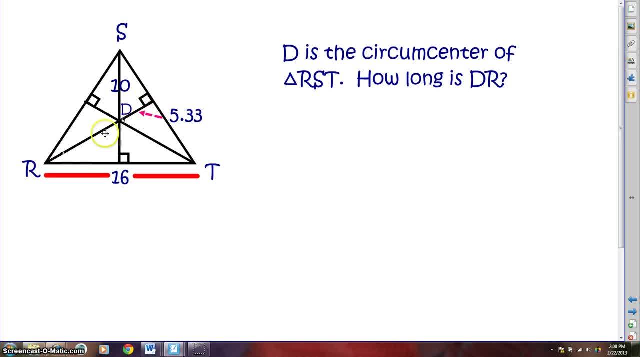 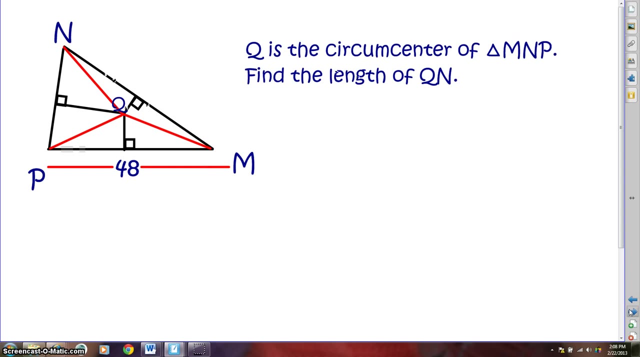 we're supposed to find dr. dr is the same length as ds. dt is also that same length. So since ds was 10,, that means dr is 10, and so is dt. We can use that to make a little bit more complicated question. 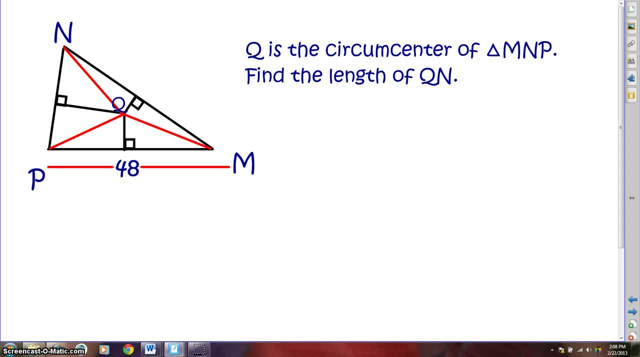 Again, if we remember how it was formed, we're supposed to find the length of qn. This time we don't know any of those lengths that go from the circumcenter out to the vertex, So that means we need to use some other information to calculate them. 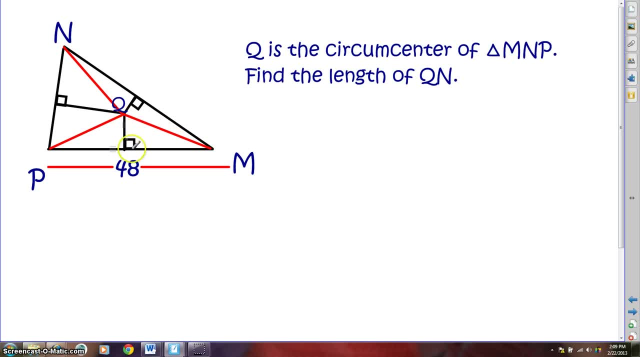 So, for instance, if we know that this was made with the perpendicular bisector, this whole side was 48. That means that this part over here is 24, and we have a right triangle. It looks like we're also missing a piece of information over here. 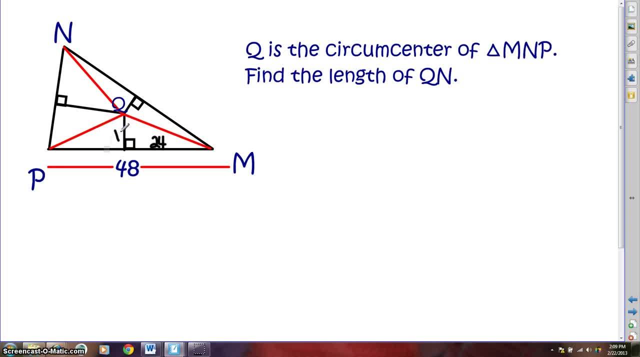 So if we say that this little segment here was 10, we'll have to add that We're missing a piece of information. If we want to find the length of qn, it's going to be the same as qm. So if we use the Pythagorean theorem on this right triangle, 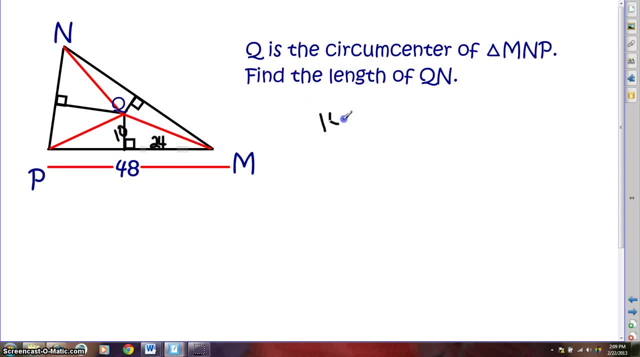 we know the two legs. So 10 squared plus 24 squared is going to equal qm squared, Which would make that 26. If we use our Pythagorean theorem to calculate that, Alright, so this segment here, qm, would be 26,. 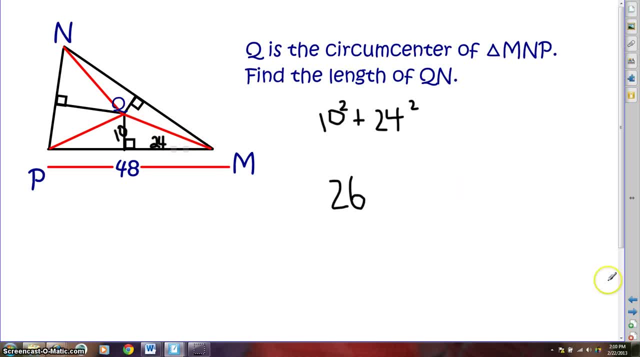 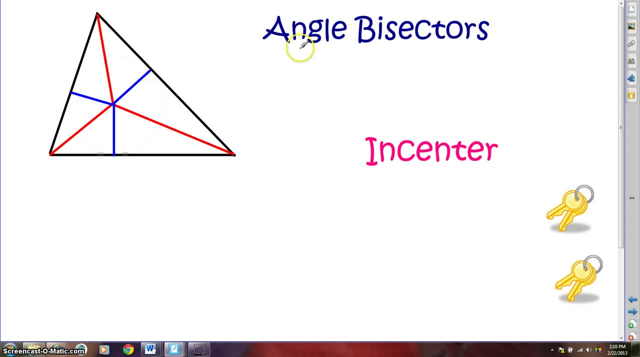 which means qn would have the same length. And that's when we're using the circumcenter. The second point of concurrency: the incenter is made by using the angle bisectors, which means each one of our angles of our triangle is split in half. 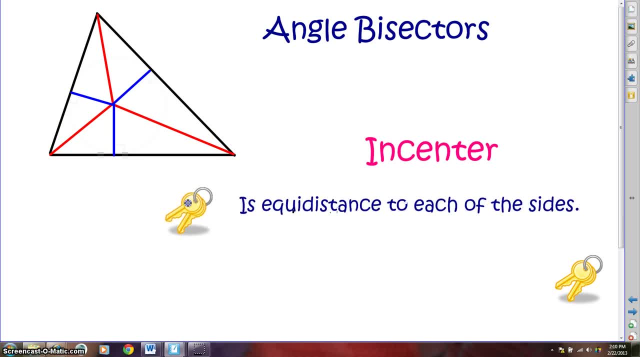 The incenter, its special characteristics- is equidistant to each one of the sides, which means for the incenter we can actually put a circle inside. So if we use the incenter and when we do that, we need to remember that. 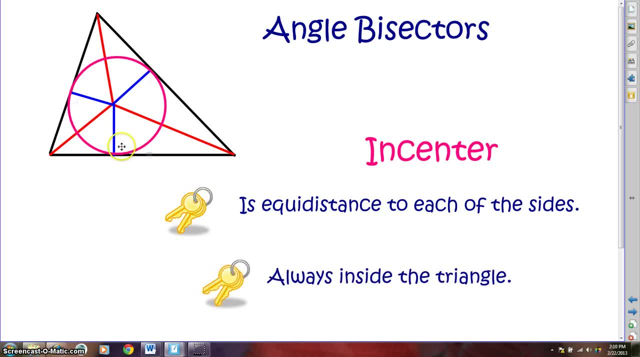 it's always going to be inside the triangle And if we're going to use the equid, if it's equidistant, that means each one of these as we connect, it has to be to be equidistant. they have to each be a right angle. 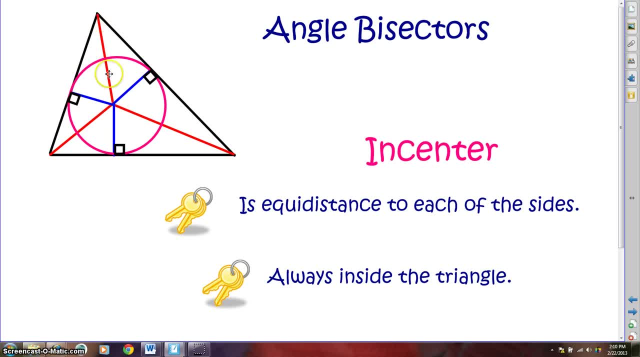 or they have to be perpendicular to the side. Alright, so the angle bisectors were what was in red right. If we go from the incenter to each one of the sides at a perpendicular, each one of these is going to be congruent. 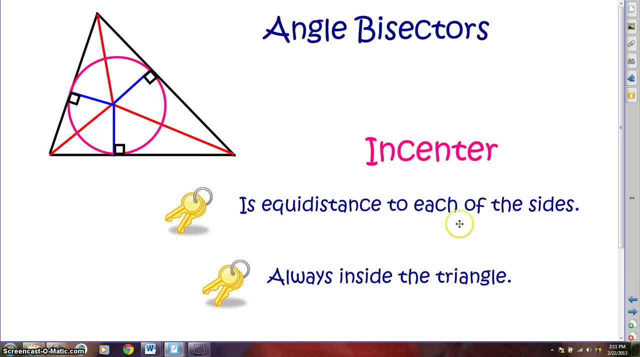 The incenter is always inside. The circumcenter moved around and the incenter is always inside. And acute triangles: the point of concurrency is always inside And the incenter is always inside the triangle. Alright, so let's take a look at what something like this would look like. 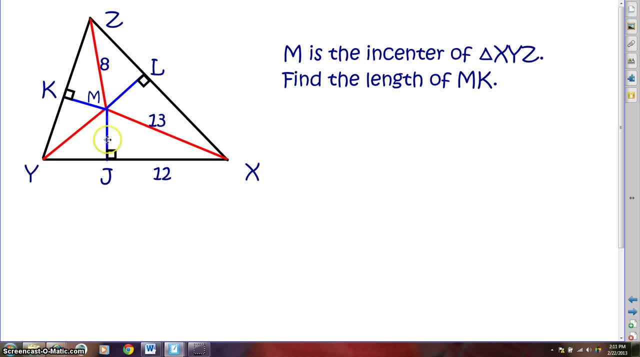 Alright, we know that m is the incenter, so it was made. with the angle bisectors We're supposed to find the length of mk. Each one of these blue segments up here is going to have the same length. So if we use this triangle here, 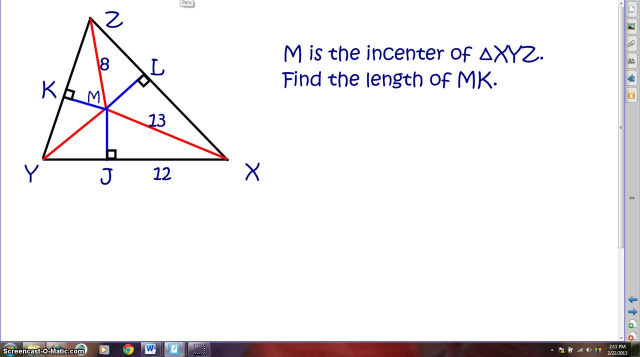 that means that 13 squared minus 12 squared is going to give us mj, and mj and mk are going to be the same. So, using our Pythagorean triples, we know that mj would have to be 5, and so would mk. 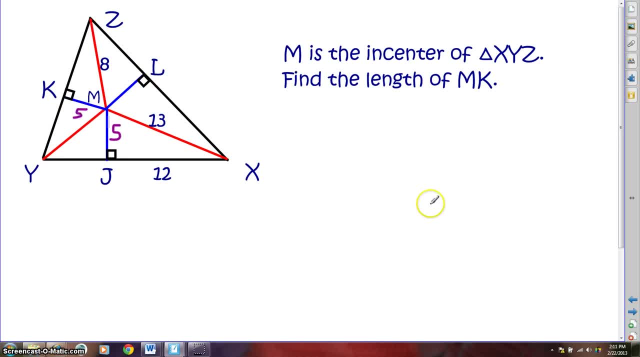 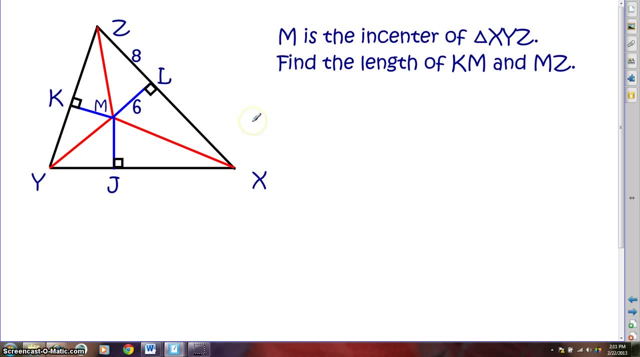 So each one of these would be 5, and so would ml. Let's take a look at another one. Alright, this time we're supposed to find the length of km and mz. km, ml and mj are all going to be the same. 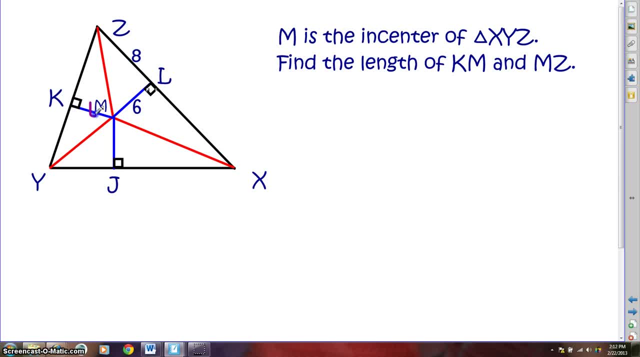 so that means, since ml was 6,, km is going to be 6, and so is mj, So km is 6.. And then to find mz, this is a right triangle, so that's one of our Pythagorean triples. 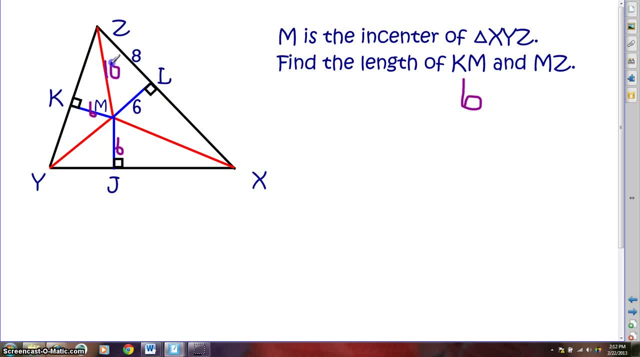 That's our 3,, 4, 5 in disguise. So mz would have a length of 10.. So km is 6, mz is 10.. Alright, so we've looked at the circumcenter which was made with the perpendicular bisectors. 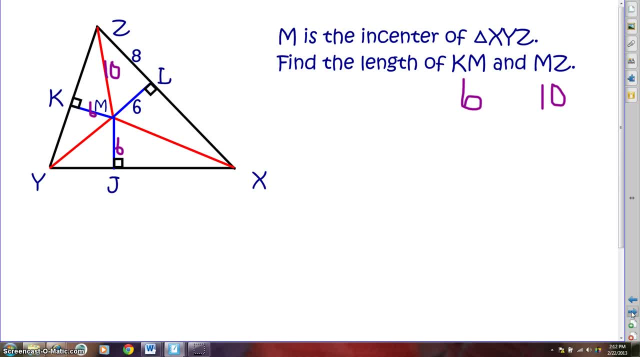 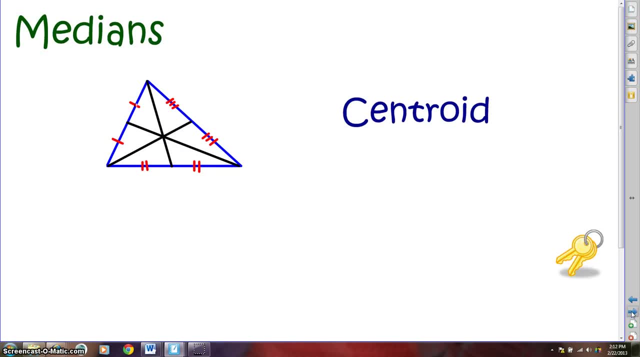 That point of concurrency is equidistant to the vertices. The in-center is made using the angle bisectors and it's equidistant to each one of the sides. Our third one is made using the medians, If you remember what a median is. 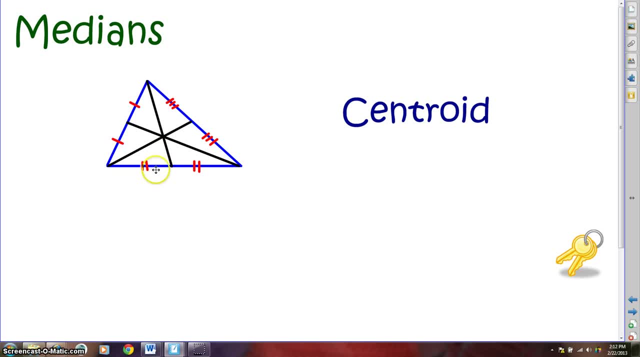 a median starts at the vertex and it connects to the midpoint of each side. Alright, so the perpendicular bisectors would go through that same point, but they would be perpendicular and would not necessarily have to go through the vertex. The median does. 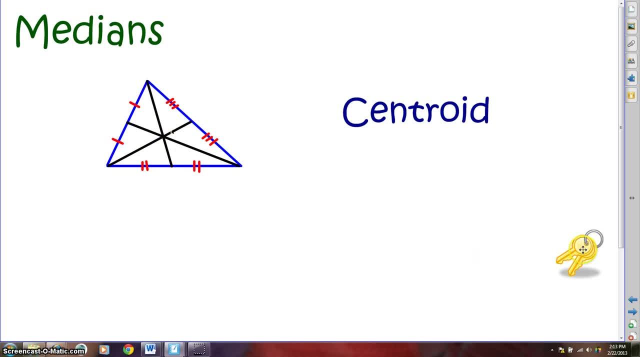 The median starts at the vertex and it connects to the midpoint And where those three cross, that's called the centroid. And the centroid is located two-thirds of the length of the median starting from the vertex. So if we know the length of the median, 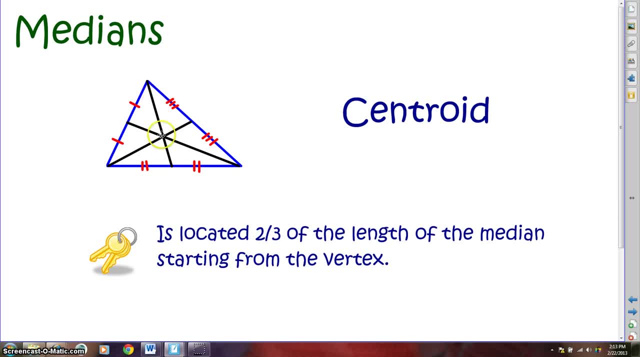 we multiply that by two-thirds, that gives us this longer segment on the top. It also means that it's one-third. the length of the median is the bottom One-third and two-thirds adds together to make the entire median. So this part is one-third of the length of the median. 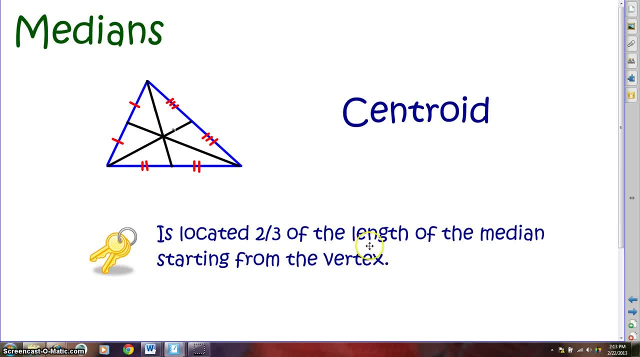 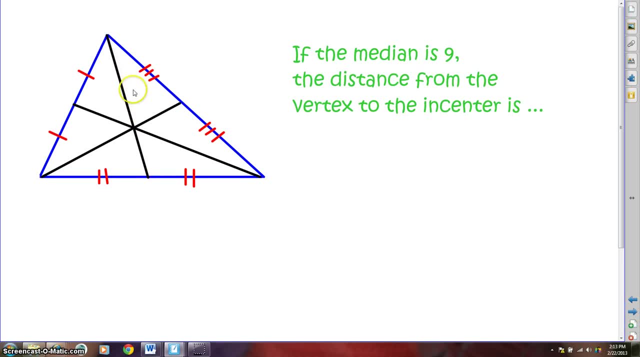 and this top part, the long part, is the median. The longer segment is two-thirds of the length of that median. So if I know, the median is nine. I want to know the distance from the vertex to the in-center. And if we remember, 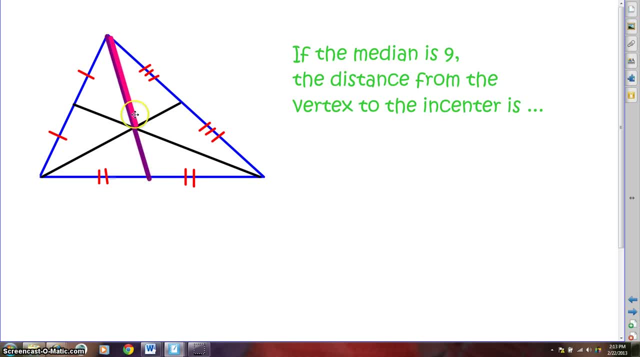 alright, the median itself alright. to find the longer segment, we take the median of nine and we multiply it by two-thirds, So that would give us a length of six, Which also means that this bottom segment down here is a third of that. 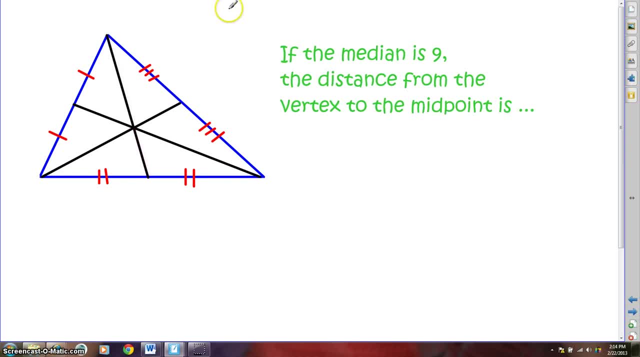 so it would be three. Alright, so if we look at that, if we just if we didn't have to know the longer segment and we were just looking for the shorter segment, the shorter segment is one-third the length of this. 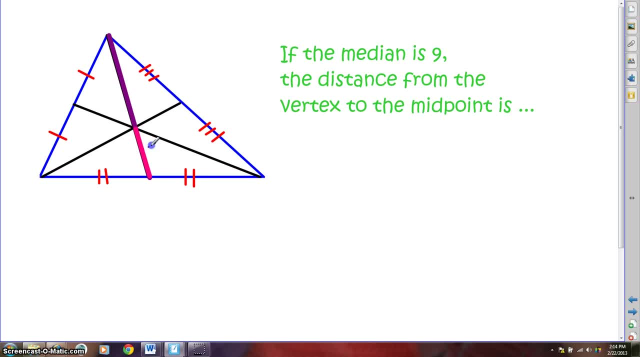 so a third of nine would be three, And again that leaves us six left over for this longer part. And then, if we look at the ratio between those two, the shorter segment is half of the longer segment. So if we look at that part,